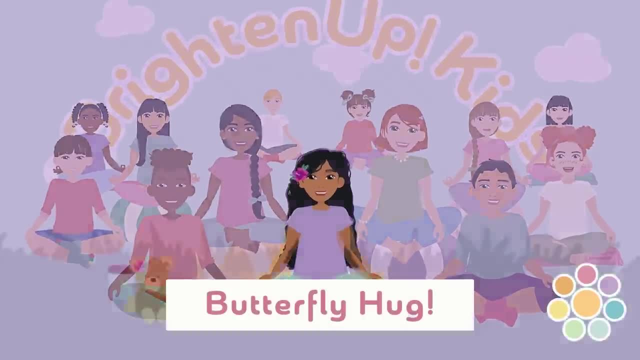 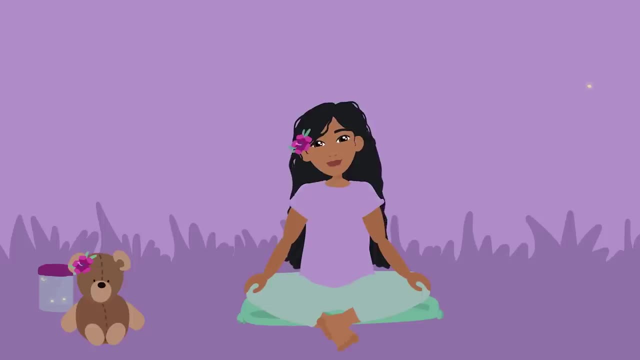 Hello there, friend, I'm so happy you're here. How are you feeling right now? It's okay to have big feelings, but they can also feel a little overwhelming, So let's help shrink them down a little bit so you can feel better. 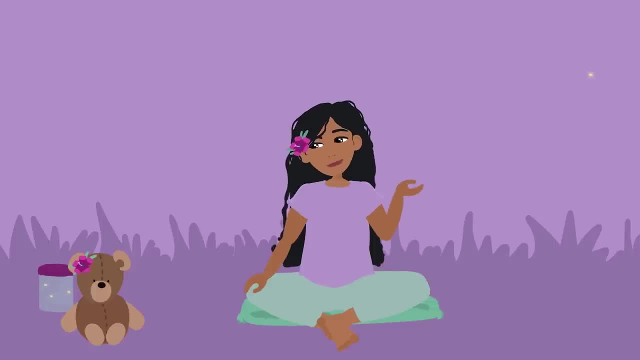 Did you know a butterfly hug could help? I know it sounds silly, but it's true. Want to try with me? Go ahead and sit in the comfortable position. Now that you're comfortable, I want you to imagine a beautiful fluttering butterfly. 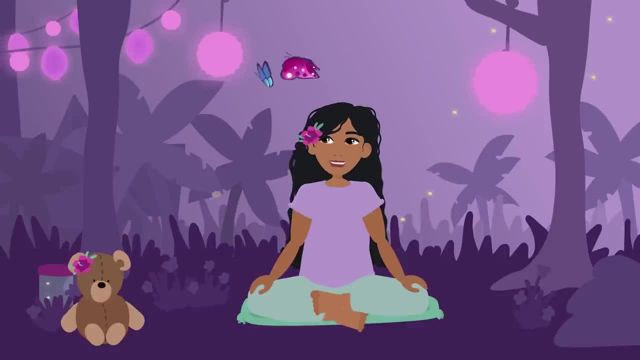 What color is your butterfly friend? Is it yellow, Pink? Does it have any fun patterns on its wings, Like polka dots Or rainbows? Maybe your butterfly has the same colors as your favorite superhero. It can be any color you want it to be. 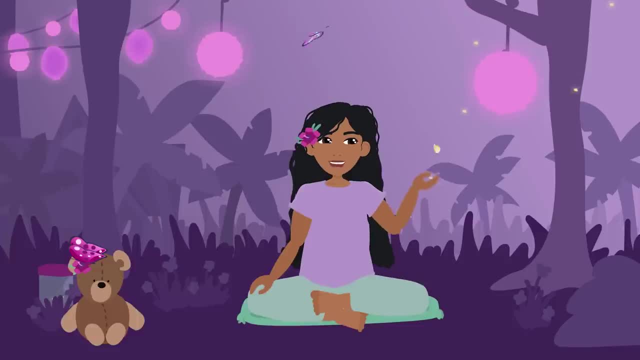 How big is your butterfly friend? Can it fit in the palm of your hand? Or maybe it's as big as a basketball? Really picture in your mind what your butterfly friend looks like And have your handsل And watch it gently flutter through the air. 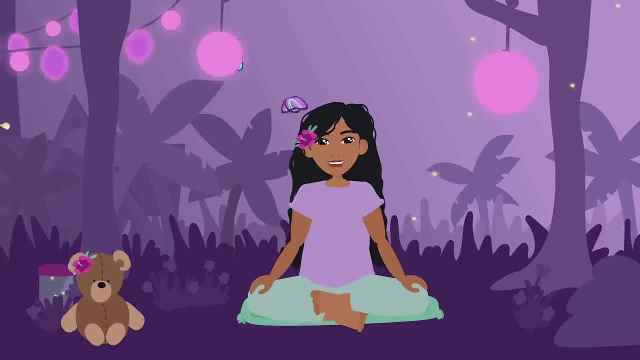 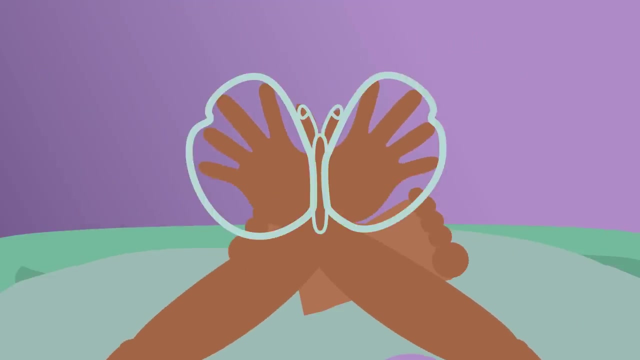 Should I wave at butterfly in bed? Now hold your hands out in front of you, with your palms facing towards you, and cross your hands so they form a butterfly. Imagine this is now the butterfly friend you've been picturing and place it on your chest, close to your heart. 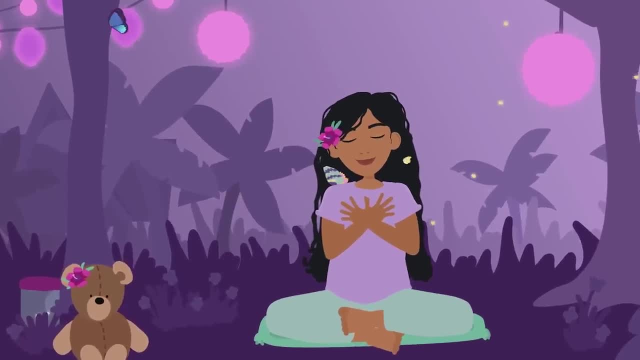 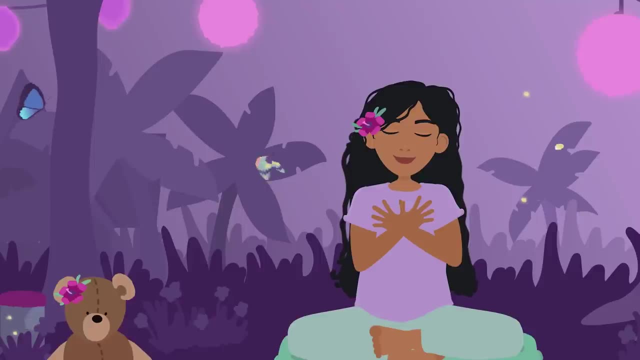 as if it's giving you a soft hug. let's take three slow, deep breaths while the butterfly gently lays on your chest. slow deep breath in through your nose and gently breathe out through your mouth. good, try to breathe in as long as you can, slowly and gently, slow deep breath in through your nose. 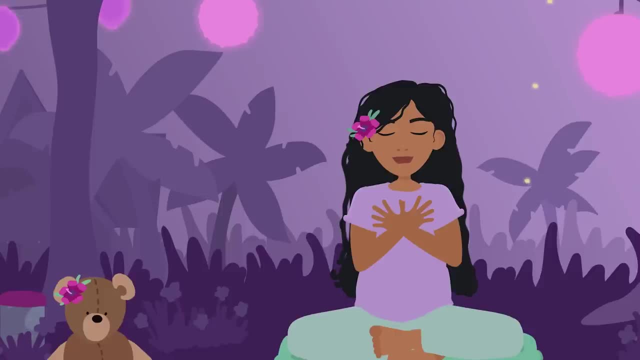 and gently breathe out through your mouth. great, one more time, slow, deep breath in through your nose and gently breathe out through your mouth. good, continue to breathe, nice and slow. did you know that your butterfly friend is actually a little magical? whenever your butterfly friend flaps its wings, it relaxes everything around it. go ahead and flap your butterfly's wings. 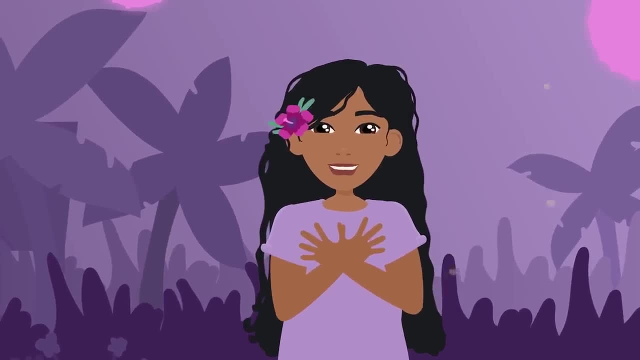 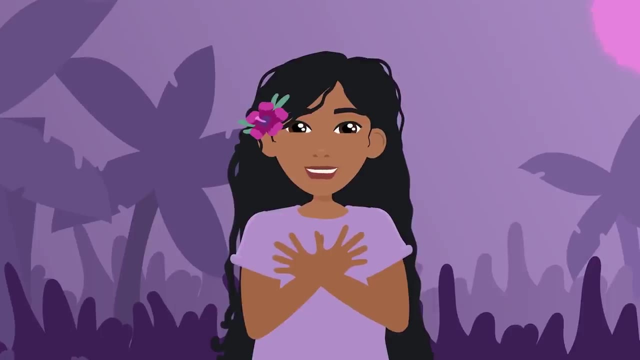 by gently tapping your hands on your chest, one at a time. tap, tap, tap, tap, tap. continue to breathe nice and slow as your butterfly friend continues to flap its wings. if it's more comfortable for you, your butterfly friend can be bigger and you can tap your shoulders instead, whichever feels best for you. 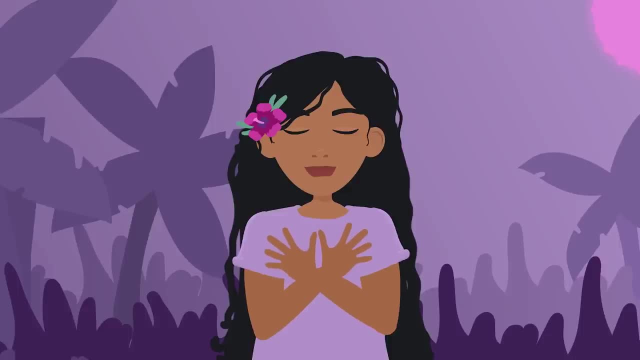 continue to slowly and gently tap, tap, tap. you can even have your butterfly flutter its wings by tapping each finger, one at a time, on each side, like a butterfly, and now the other side. you can switch between tapping and fluttering whenever you want, if you think you might have transferred too quickly, or好了. 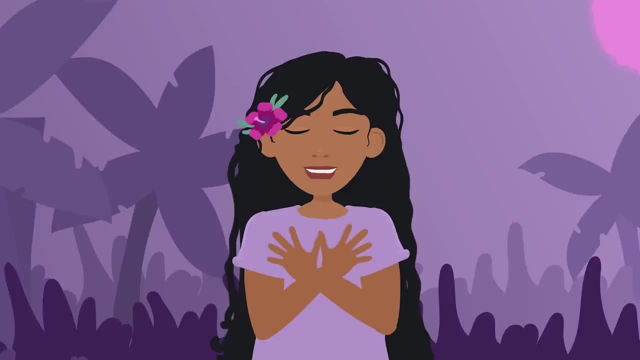 this already happened. come straight to the point. click on a fewacionaldroidscom from live��계 and you got all the solid stacks ofatin-sline bands. And now the other side. you can switch between tapping and fluttering whenever you want positive affirmations, while your butterfly friend continues to tap its.